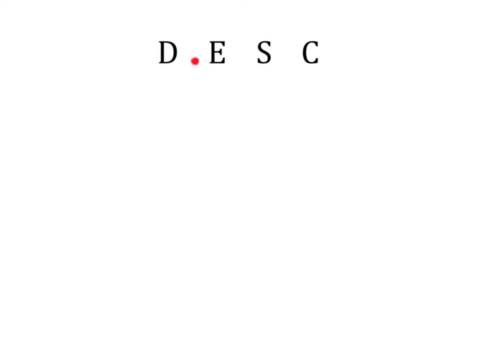 going to say this phrase: Use your desk So D-E-S-K. So desk helps us remember the process that we're going to follow every time we have a word problem. So the D in desk is going to stand for define your variables. I want to know in words, what does X represent and 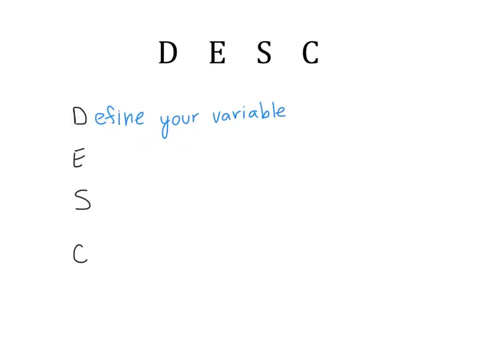 what does Y represent in terms of your word problem? The E in desk represents equation, because after we define our variables, we're going to make an equation, Then we're going to do the S, which is to solve. So we're going to solve our equation, for whatever. 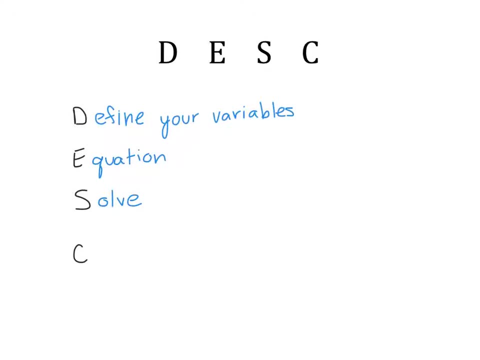 they're asking for. And then the C in desk is to write a complete sentence. So we're always going to answer these word problems with a complete and thorough sentence. So every time I say use your desk, it means define your variables, make an equation, solve and then complete sentence. 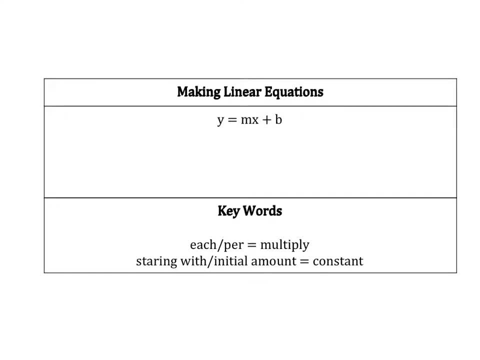 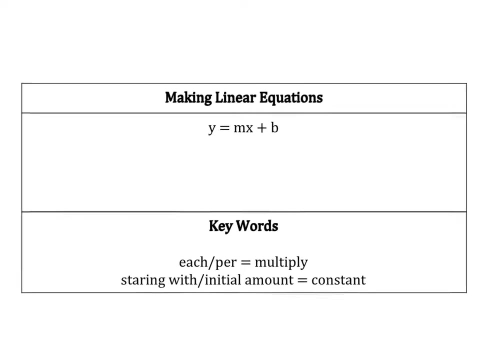 Okay, so today, like I said, we're going to be making linear equations from real life examples. So we're going to be doing this with Y equals M-X plus B, our slope-intercept form. So it is kind of useful to know what some of these different variables might represent. 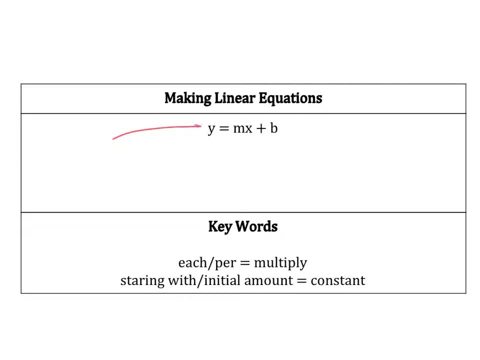 So let's start with Y. So Y is always going to be what we are trying to find, What we're trying to find, And you also might call this, or you might hear it called, the dependent variable- Dependent, Because this outcome is going to depend on some other input. 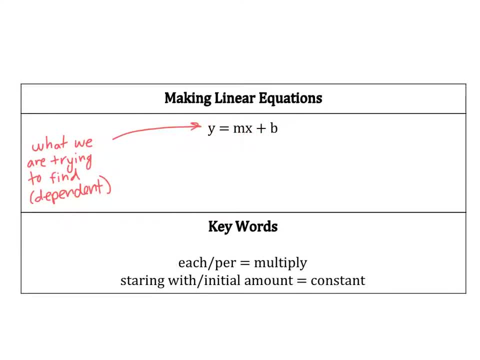 So our Y is always going to depend on what we choose for X, Which brings us to X. So X is what we choose, And we call this the independent variable, And it can be what we choose or what we change. So this is the thing that we pick and this is what we get out of it. 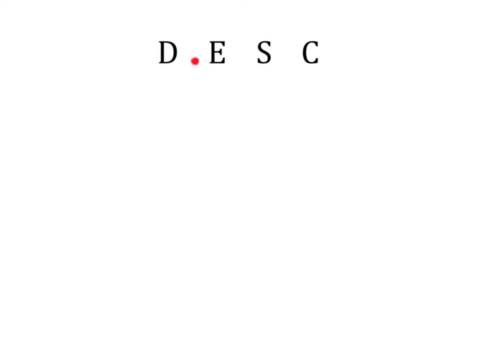 going to say this phrase: Use your desk So D-E-S-K. So desk helps us remember the process that we're going to follow every time we have a word problem. So the D in desk is going to stand for define your variables. I want to know in words, what does X represent and 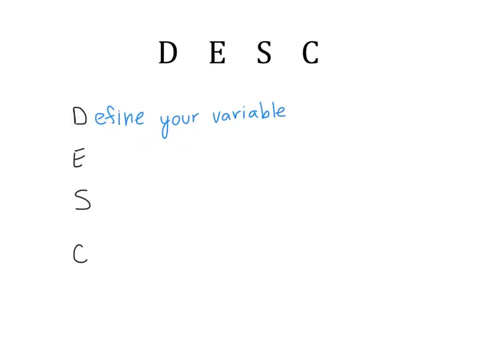 what does Y represent in terms of your word problem? The E in desk represents equation, because after we define our variables, we're going to make an equation, Then we're going to do the S, which is to solve. So we're going to solve our equation, for whatever. 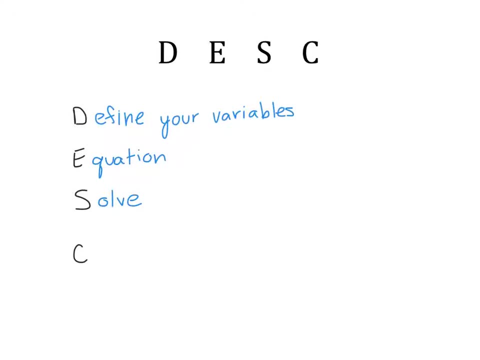 they're asking for. And then the C in desk is to write a complete sentence. So we're always going to answer these word problems with a complete and thorough sentence. So every time I say use your desk, it means define your variables, make an equation, solve and then complete sentence. 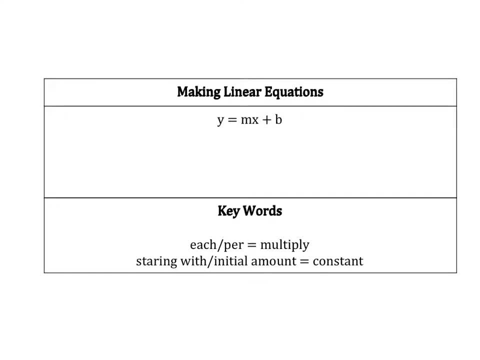 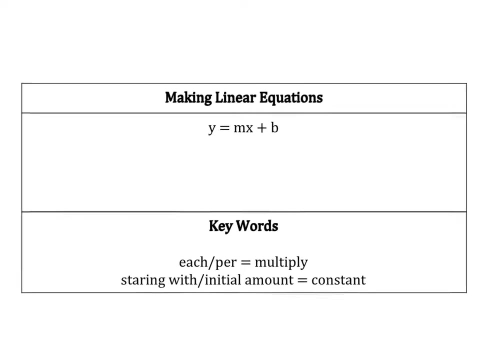 Okay, so today, like I said, we're going to be making linear equations from real life examples. So we're going to be doing this with Y equals M-X plus B, our slope-intercept form. So it is kind of useful to know what some of these different variables might represent. 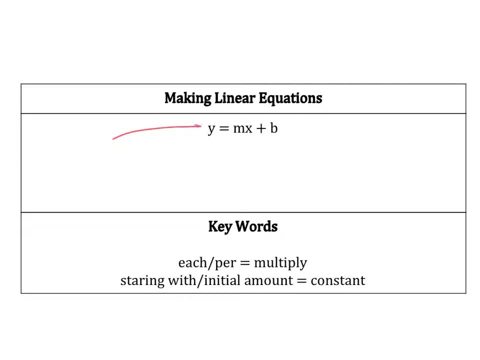 So let's start with Y. So Y is always going to be what we are trying to find, What we're trying to find, And you also might call this, or you might hear it called, the dependent variable- Dependent, Because this outcome is going to depend on some other input. 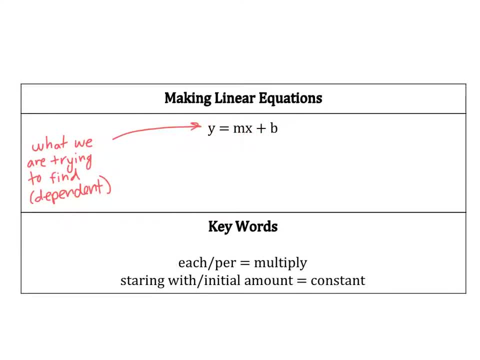 So our Y is always going to depend on what we choose for X, Which brings us to X. So X is what we choose, And we call this the independent variable, And it can be what we choose or what we change. So this is the thing that we pick and this is what we get out of it. 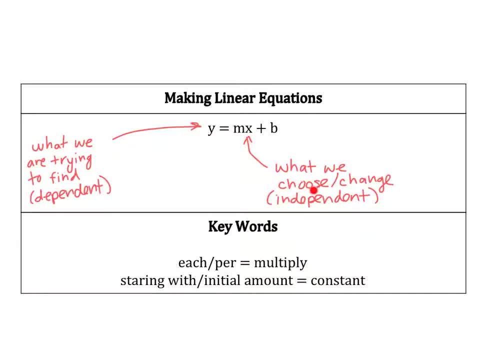 So this is why this is the independent variable. We can pick whatever we want. Our Y will depend on what our X is, So that's why they call it the dependent variable. Now we still have M and B, So these are going to be things that we can pull out of our word. 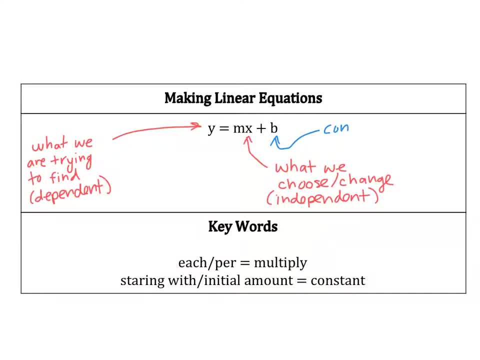 problem. So B is what we call a constant. So a constant is something that never changes. So you can think of it like that. And in these types of word problems, our constant is going to be our starting value. So anytime we're starting with a certain amount, that's going. 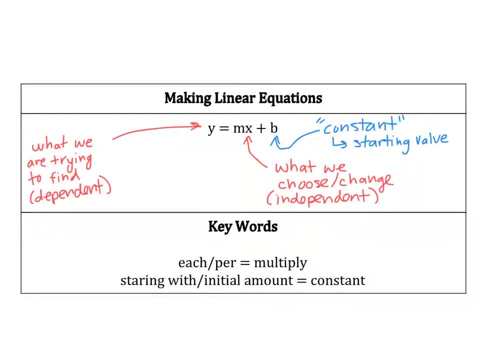 to be our constant. So we're going to put that value right here Now. M. as we know, M represents slope, which is change of Y over change of X. In word problems. M is going to be how much we change Which. 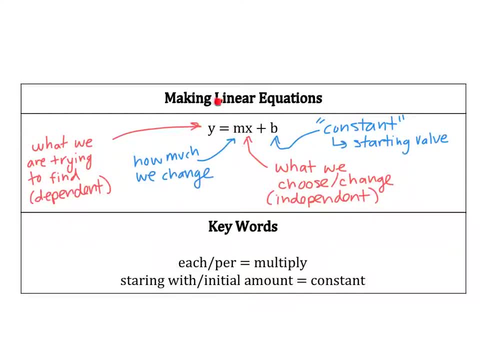 kind of makes sense for the slope, because slope is how much you change going from one point to the next. So we can kind of use these guidelines to help us look at words and translate them into a math equation. Now a few other key words that it might be useful to know is anytime you see the word 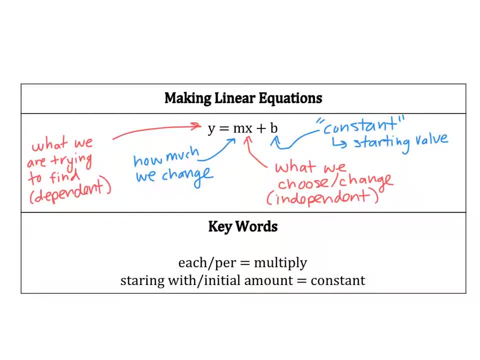 each or per, like Ms Ruddy has 20 students per class. that is going to tell us to multiply those values And anytime you see the words starting with or initial amount, that is going to represent that constant value which goes where our B value is. So those are just little. 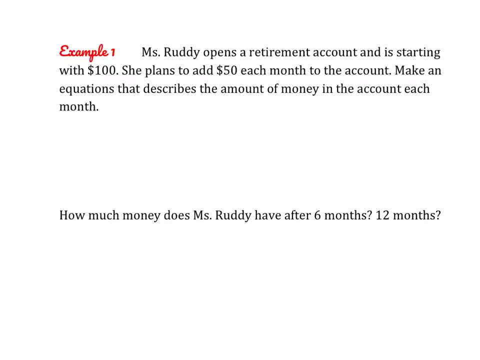 hints that we might use to help us. Okay, so let's give one of these a try. So we're going to start with our B, So we're going to use our desk, but before we do that, we're going to read the equation and I'm going. 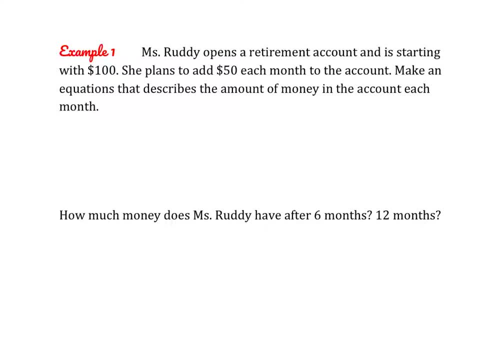 to highlight some important information. So Ms Ruddy opens a retirement account and is starting with $100. So I go to a bank and I want to start saving for retirement. So I open a bank account and this is how much I'm starting with. She plans to add $50 each month to the account. So this is how much. 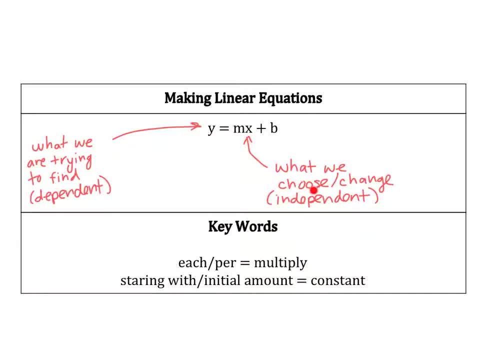 So this is why this is the independent variable. We can pick whatever we want. Our Y will depend on what our X is, So that's why they call it the dependent variable. Now we still have M and B, So these are going to be things that we can pull out of our word. 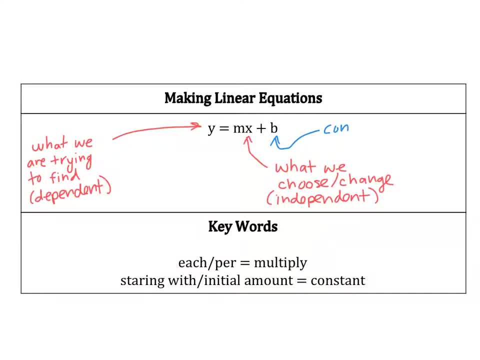 problem. So B is what we call a constant. So a constant is something that never changes. So you can think of it like that. And in these types of word problems, our constant is going to be our starting value. So anytime we're starting with a certain amount, that's going. 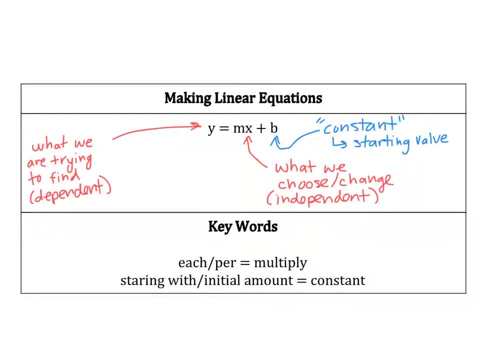 to be our constant. So we're going to put that value right here Now. M. as we know, M represents slope, which is change of Y over change of X. In word problems. M is going to be how much we change Which. 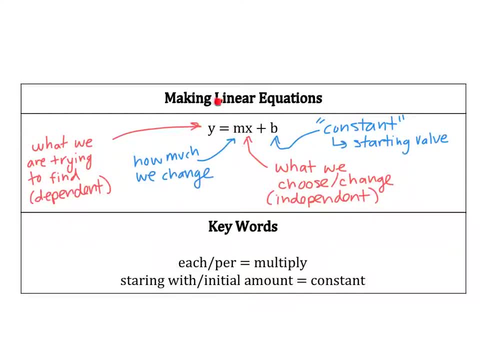 kind of makes sense for the slope, because slope is how much you change going from one point to the next. So we can kind of use these guidelines to help us look at words and translate them into a math equation. Now a few other key words that it might be useful to know is anytime you see the word 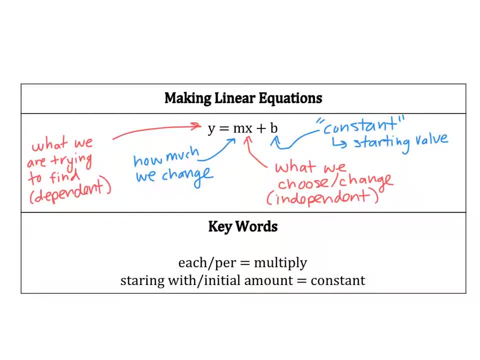 each or per, like Ms Ruddy has 20 students per class. that is going to tell us to multiply those values And anytime you see the words starting with or initial amount, that is going to represent that constant value which goes where our B value is. So those are just little. 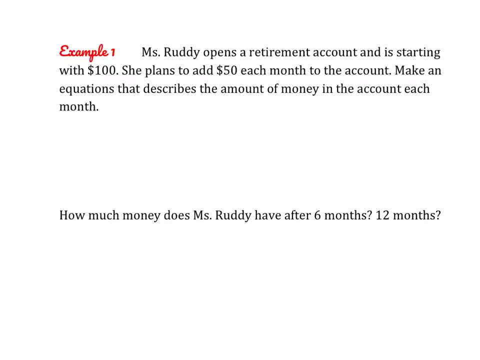 hints that we might use to help us. Okay, so let's give one of these a try. So we're going to start with our B, So we're going to use our desk, but before we do that, we're going to read the equation and I'm going. 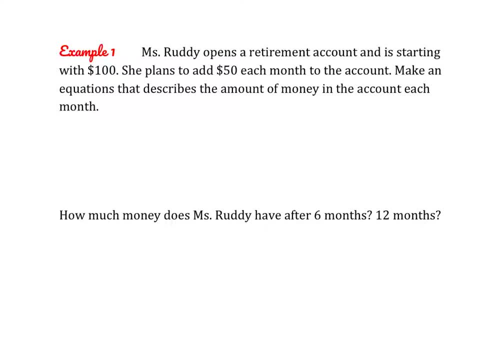 to highlight some important information. So Ms Ruddy opens a retirement account and is starting with $100. So I go to a bank and I want to start saving for retirement. So I open a bank account and this is how much I'm starting with. She plans to add $50 each month to the account. So this is how much. 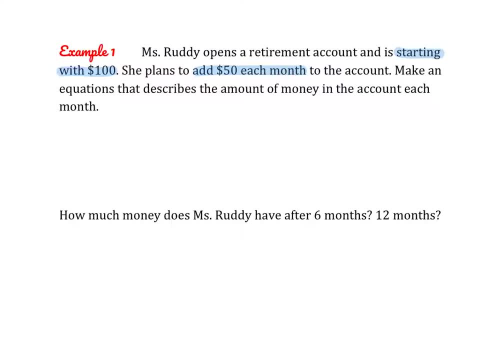 my account is going to change. So this is how much my account is going to change each month. So we want to make an equation that describes oops, that describes the amount of money in the account each month. So the first thing we're going to do, again, the first letter of desk is D, which stands for 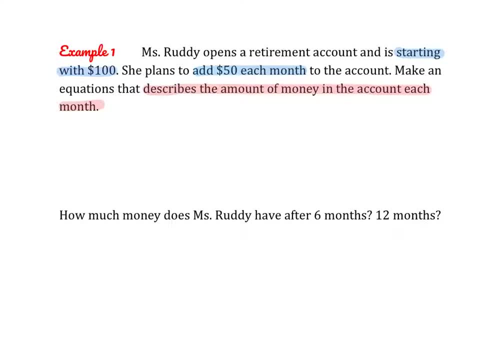 defining your variables. So I want to know what does X represent and what does Y represent? So remember, X represents the only thing that we can change. So, once again, our Y represents the one that will represent our pay. So what we're going? 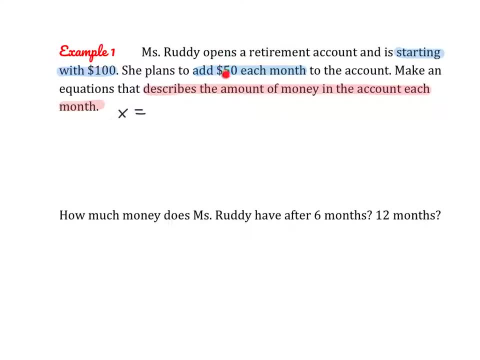 to do is we're going to want to find the number of times we're going to get paid in this equation. So we can't change the starting amount. we can't change how much money Ms Ruddy is adding each month, but we can change which month it is or how many months have gone by. So 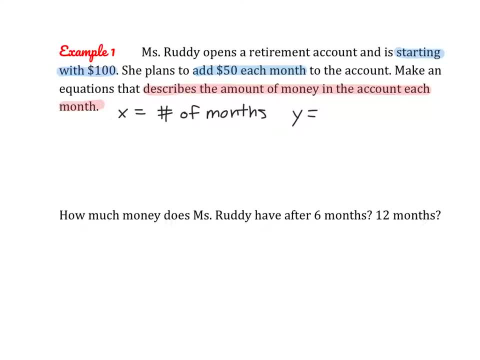 the number of months is what we're going to pick. so that's our X value is the number of months. Now, remember, our Y value is always going to represent what we're trying to find and in the account, so that's what our Y value is going to equal the money in the 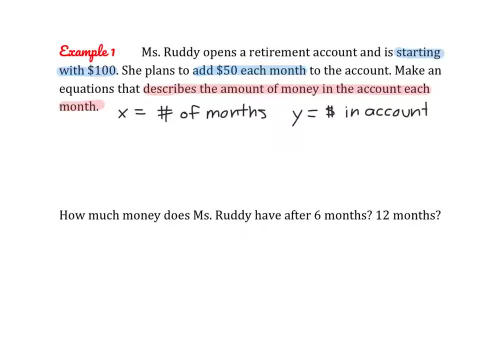 account. now, of course, the amount of money in the account is going to depend on how many months has gone by. so that's why X is the independent and Y is the dependent, the. so to repeat that, the amount of the money in the account depends on how many months has gone by. so this is the independent variable and 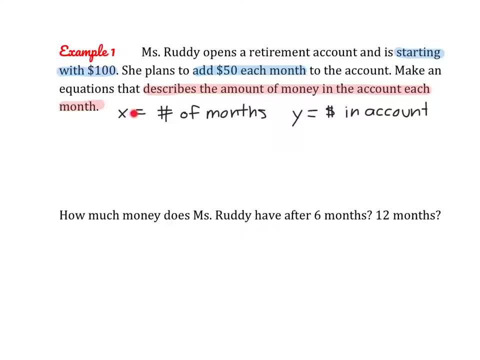 this is the independent variable. so we just finished the D and desk. we defined X and Y. we defined our variables. now the E and S tells us to make an equation. so we know we're going to use: Y equals MX plus B. now let's think about what our M 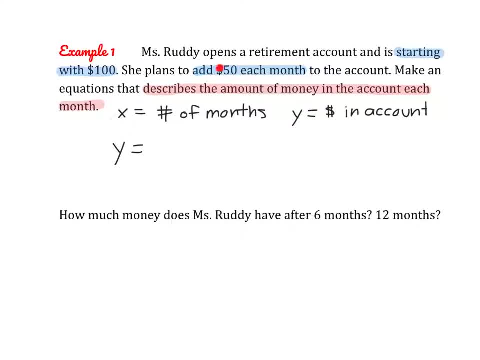 value is. so remember, M is how much something is changing. so here I see: oh, we're adding $50 each month. I also want to remind you: each tells us to multiply, so we have 50 multiply by months, which is represented by X. so 50 times X is 50 X. now I want to remind. 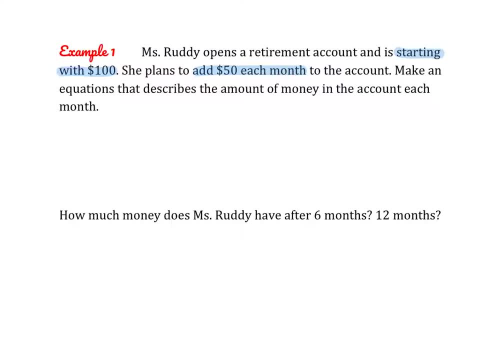 my account is going to change. So this is how much my account is going to change each month. So we want to make an equation that describes oops, that describes the amount of money in the account each month. So the first thing we're going to do, again, the first letter of desk is D, which stands for 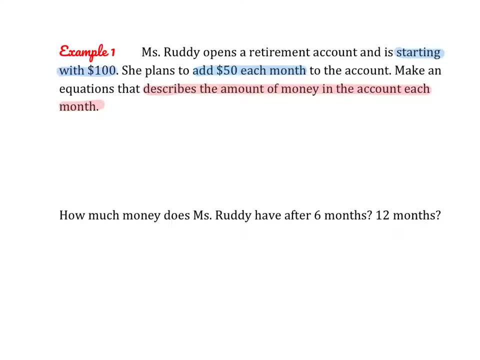 defining your variables. So I want to know what does X represent and what does Y represent? So remember, X represents the only thing that we can change. So we can't change the starting amount. We can't change how much money Ms Ruddy is adding. 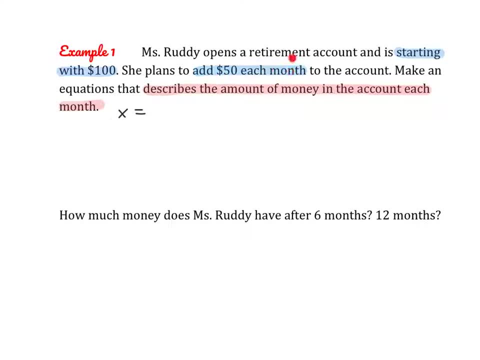 each month, but we can change which month it is or how many months have gone by. So the number of months is what we're going to pick. so that's our X value is the number of months. Now, remember, our Y value is always going to represent what we're trying to find and we 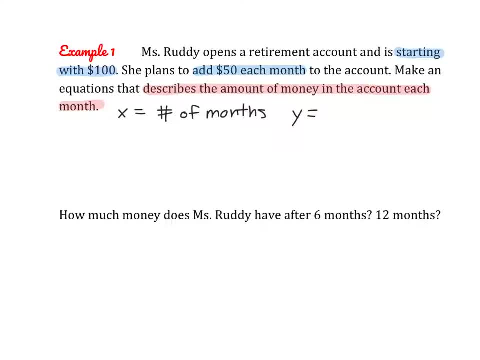 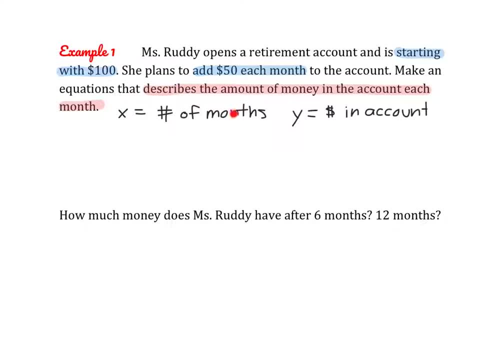 Now, of course, the amount of money in the account is going to depend on how many months has gone by. So that's why X is the independent and Y is the dependent. So to repeat that, the amount of the money in the account depends on how many months has gone by. So this is. 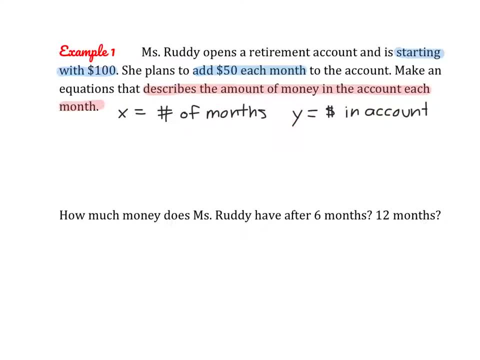 the dependent variable and this is the independent variable, and this is the independent variable, independent variable. So we just finished the D and desk. We defined X and Y, We defined our variables. Now the E and desk tells us to make an equation. So we know we're going to use Y equals. 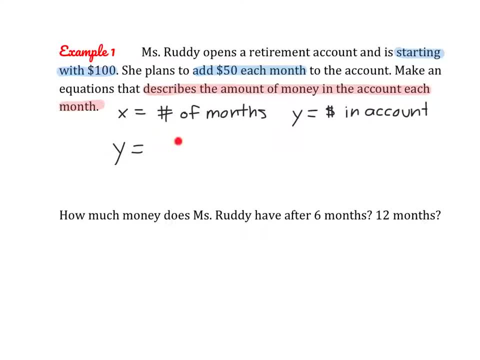 MX plus B. Now let's think about what our M value is. So remember, M is how much. something is changing. So here I see: oh, we're adding $50 each month. I also want to remind you- each tells us to. 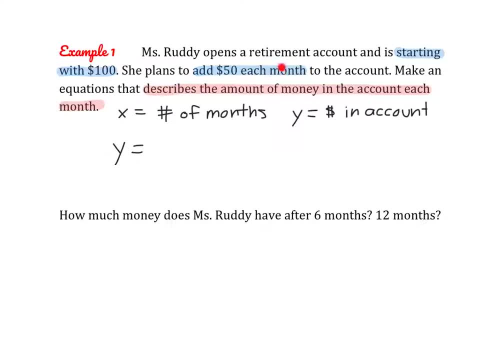 multiply. So we have 50 multiplied by months, which is represented by X. So 50 times X is 50X. Now I want to remind you guys also that that B value is always going to be our starting amount, And it says that Ms Reddy is starting with $100.. So we say plus 100. And this is the equation that 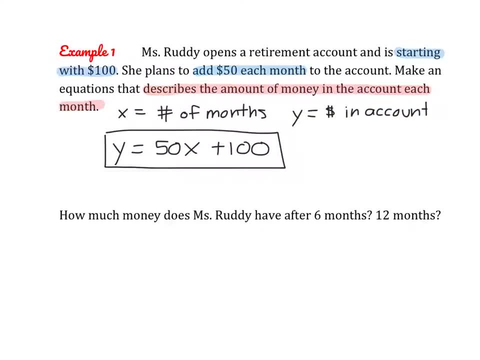 we can use to find the amount of money in the account for however many months she's been saving. So this kind of makes sense, right? Let's say I'm saving for three months, I'm going to do 50 times three because I've gone to the bank three times and put $50 in. But of course I also have that. 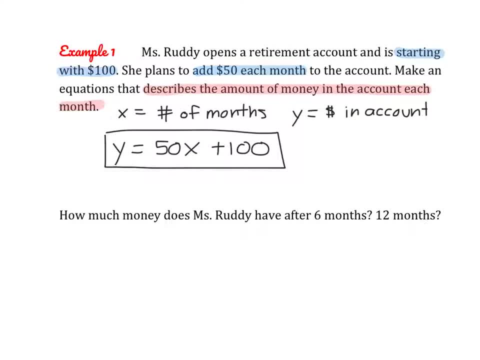 starting amount of 100.. Now you might think, well, why can't I just solve it like that? Because if you're looking way down the line, let's say I'm thinking, maybe 50 months from now you're not going to want to sit there and say 50 plus 50 plus 50 plus 50 that many times. So if we can make an, 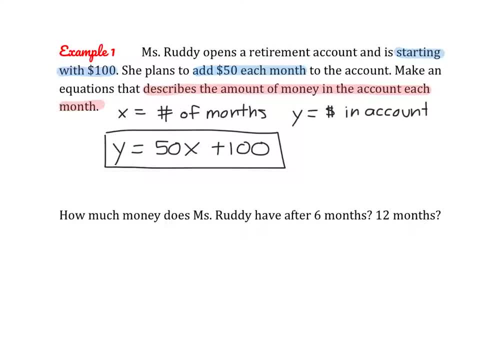 equation to represent that then we're going to have a starting amount of money in the account for the amount of money. It saves us a lot of time. So now let's do the S in DESK. We want to solve what they're asking. So down here they're asking: how much money does Ms Reddy have after six months? 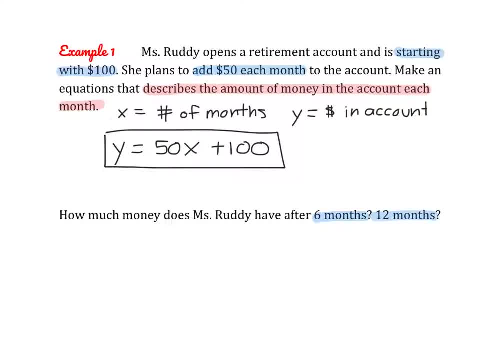 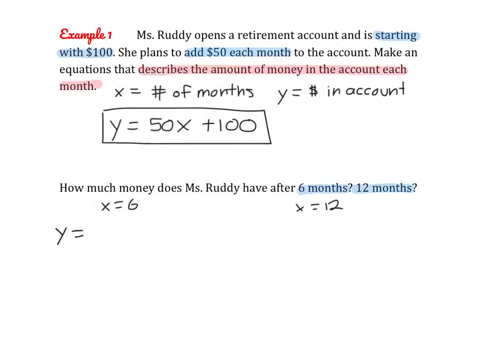 and then after 12 months. So remember, months is represented by X. So we're going to substitute X equals 6 and X equals 12 to help us find our Y value, which will represent how much money. So let's substitute X equals 6.. 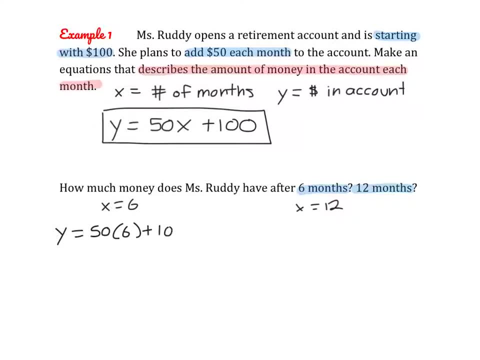 So we have 50 times 6 plus 100.. 50 times 6 is 300 plus 100 is 400.. And now we're going to do the same thing, except X will equal 12.. So 50 times 12 plus 100.. 50 times 12 is 600 plus 100 is 700.. So this is really. 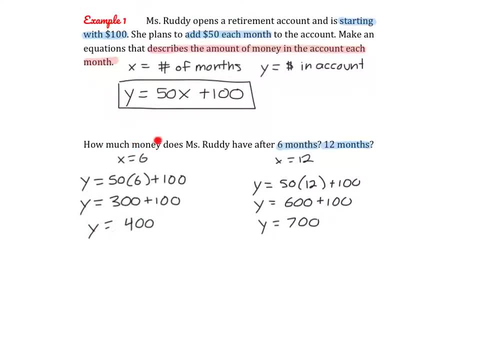 nice, We have a correct answer. However, if someone asked how much money does Ms Reddy have after six months and you said Y equals 400, that doesn't really make sense in terms of a real life problem. So we're going to want to try to write this answer as a complete and thorough sentence. 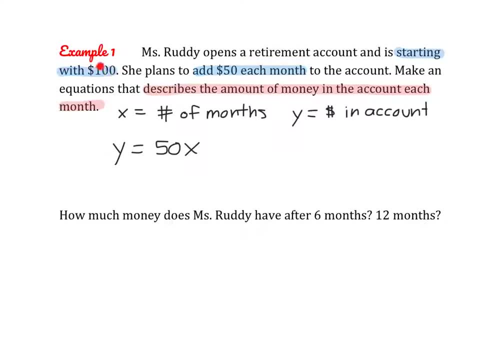 you guys also that that B value is always going to be our starting amount and it says that miss ready is starting with $100. so we say plus 100 and this is the equation that we can use to find the amount of money in the account for. 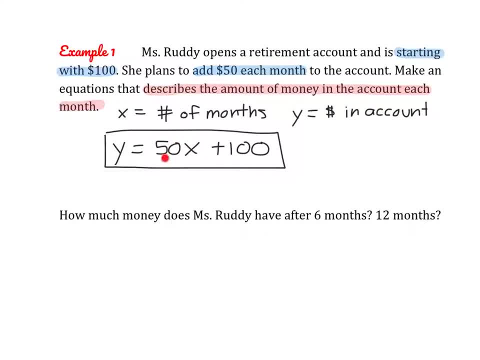 however many months she's been saving. so this kind of makes sense, right? let's say I'm saving for three months, I'm going to do 50 times three because I've gone to the bank three times and put $50 in. but of course I also have that starting. 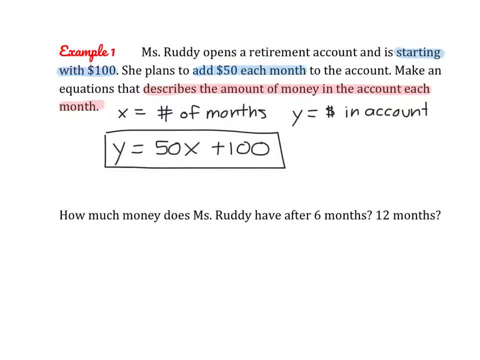 amount of 100. now you might think why can't I just solve it like that? because if you're looking way down the line, let's say I'm thinking maybe 50 months from now you're not going to want to sit there and say 50 plus 50 plus 50 plus 50. 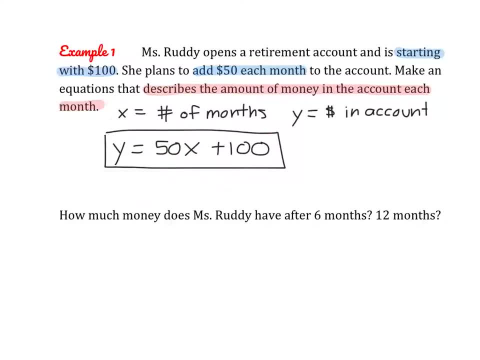 that many times. so if we can make an equation to represent the amount of money, it saves us a lot of time. So now let's do the S in DESK. We want to solve what they're asking. So down here they're asking: how much money does Ms Reddy have after 6 months and then after 12 months? 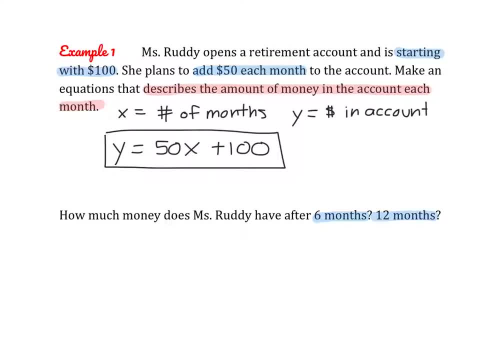 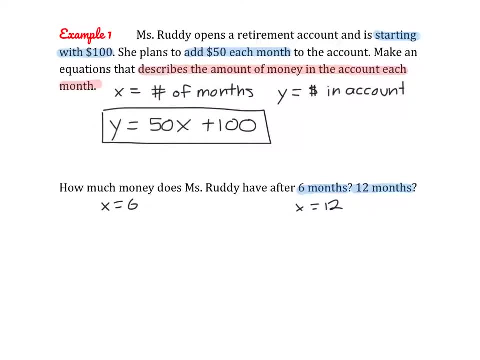 So remember, months is represented by X. So we're going to substitute X equals 6 and X equals 12 to help us find our Y value, which will represent how much money. So let's substitute X equals 6.. So we have 50 times 6 plus 100. 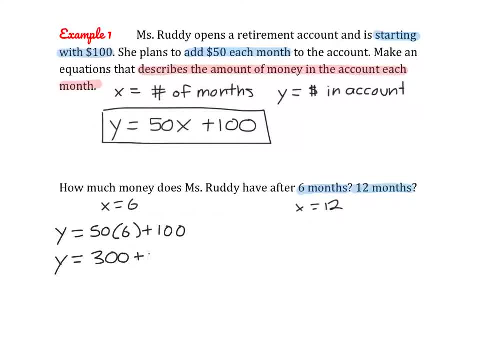 50 times 6 is 300 plus 100 is 400.. And now we're going to do the same thing, except X will equal 12.. So 50 times 12 plus 100.. 50 times 12 is 600 plus 100 is 700.. 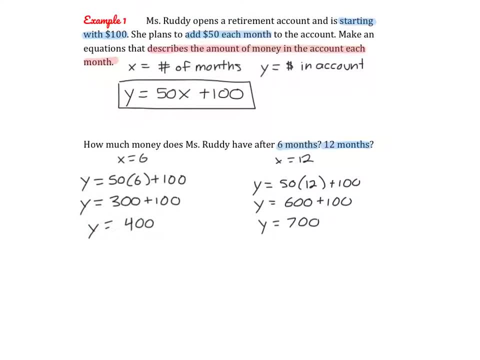 So this is really nice. We have a correct answer. However, if someone asked how much money does Ms Reddy have after 6 months and you said Y equals 400, that doesn't really make sense in terms of a real-life problem. 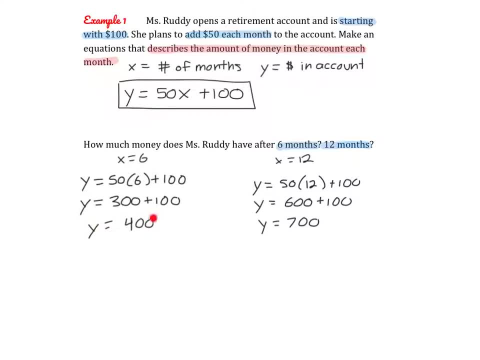 So we're going to want to try to write this answer as a complete and thorough sentence that answers the question. So how much money does Ms Reddy have after 6 months? We're going to start with after 6 months, Ms Reddy. 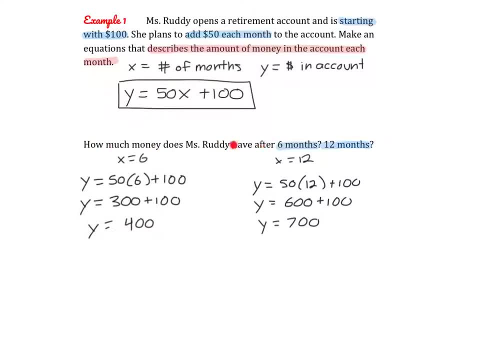 that answers the question. So how much money does Ms Reddy have after six months? We're going to start with, after six months Ms Reddy has $400.. So this is the kind of complete sentence I would expect. Let's answer that second part. 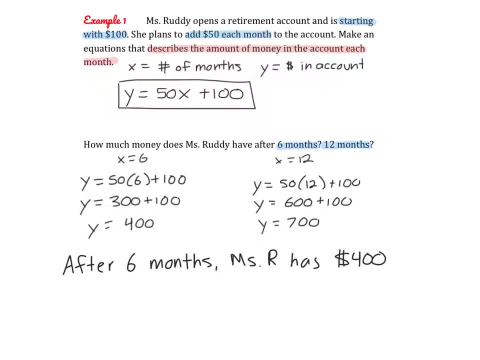 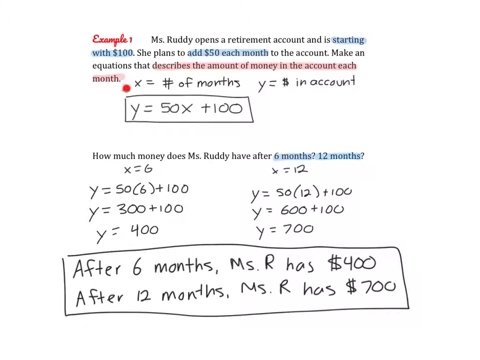 How much money does Ms Reddy have after 12 months? So we can say, after 12 months, Ms Reddy has $700.. And this is going to be our final answer. However, we need to show every step of the way. You need to define your variables. 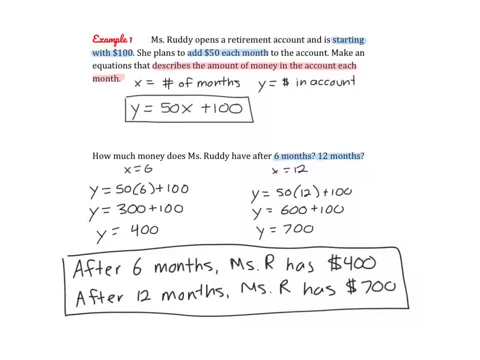 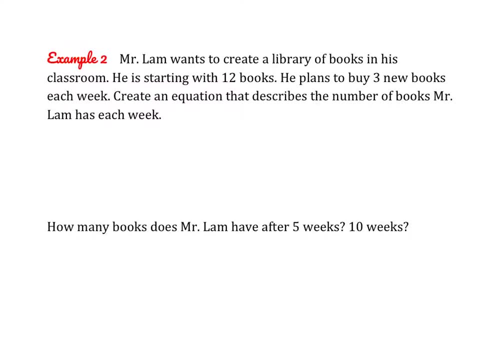 make your equation solve and write a complete sentence. Okay, let's try one more together. So here, Mr Lamb wants to create a library of books in his classroom. He is starting with 12 books. He plans to buy three new books each week. Create an. equation that describes what he's going to buy. He plans to buy three new books each week, And so he's going to start with 12 books. He plans to buy three new books each week. Create an equation that describes how much money does Ms Reddy have after 12 months. How much money does Ms Reddy have after 12 months? 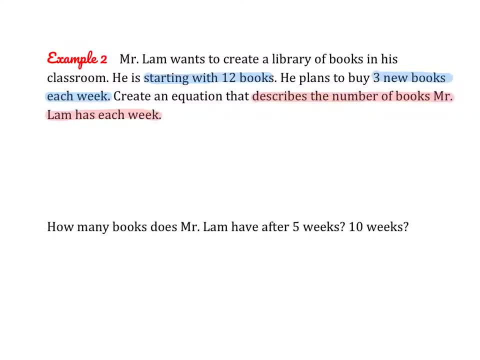 describes the number of books Mr Lamb has each week. So let's start by defining our variables. So X is going to be the thing that we control, and the only thing that we can control is the number of weeks. We can say, oh, after one week, after five weeks, after 20 weeks, it doesn't. 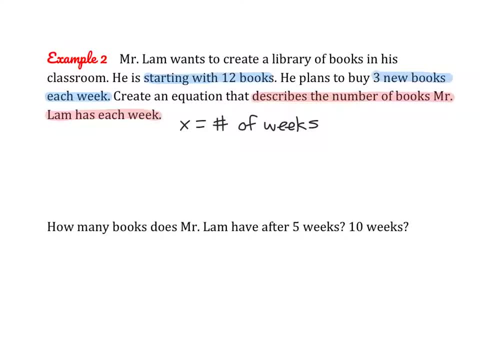 matter. So X represents the number of weeks. That's the thing that we can change. Y is always going to represent what we want to find, and they ask us to describe the number of books Mr Lamb has. So Y is going to represent the total number of books. 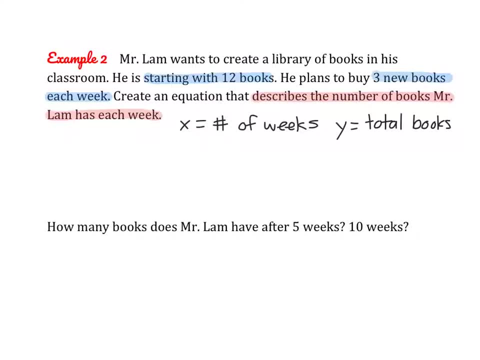 So that's the D in DESC. We are defining our variables using real words. Now we need to E make an equation, So we're going to do Y equals. So here I can see that the number of books is changing by three each week. So we can take three and multiply it by the number of weeks. 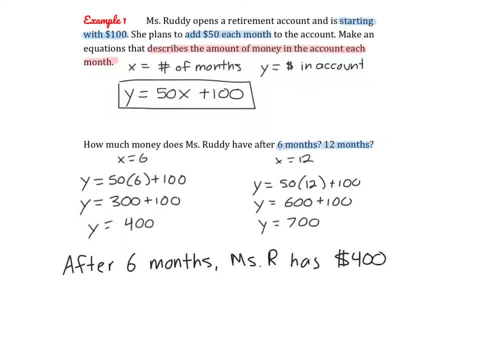 has $400.. So this is the kind of complete sentence I would expect. Let's answer that second part. How much money does Ms Reddy have after 12 months? So we can say, after 12 months Ms Reddy has $700. 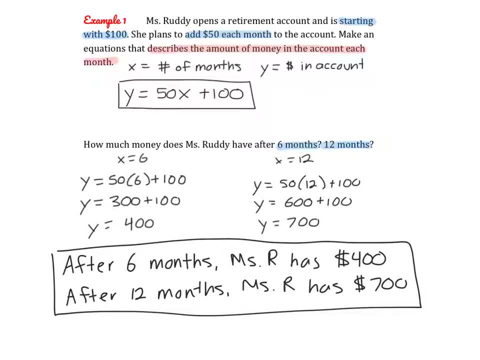 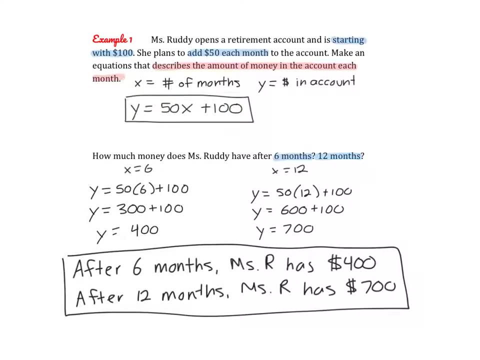 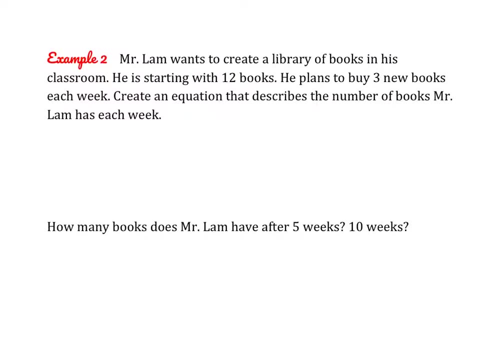 And this is going to be our final answer. However, we need to show every step of the way. You need to define your variables, make your equation solve and write a complete sentence. Okay, let's try one more together. So here, Mr Lamb wants to create a library of books in his classroom. 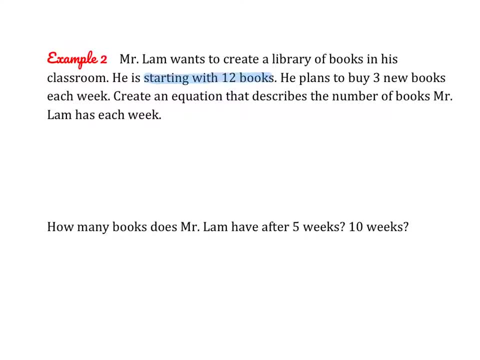 He is starting with 12 books. He plans to buy three new books each week. Create an equation that describes, Describes the number of books Mr Lamb has each week. So let's start by defining our variables. So X is going to be the thing that we control. 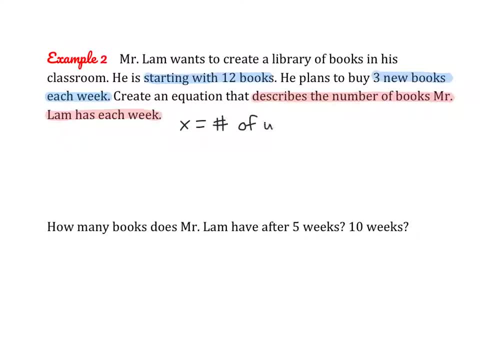 And the only thing that we can control is the number of weeks. We can say, after one week, after five weeks, after 20 weeks, It doesn't matter. So X represents the number of weeks. That's the thing that we can change. 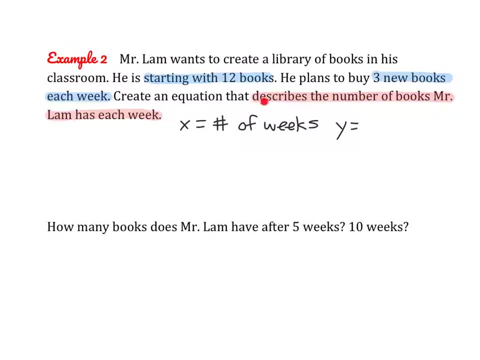 Y is always going to represent what we want to find, And they ask us to describe the number of books Mr Lamb has. So Y is going to represent the total number of books. So that's the D in desk. We are defining our variables using real words. 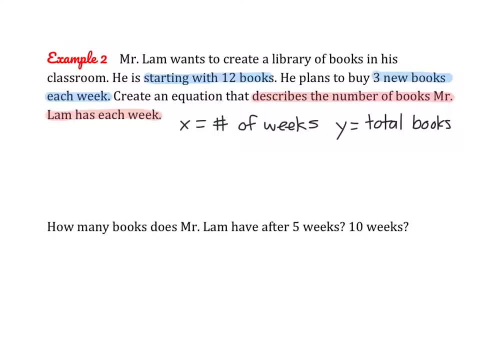 Now we need to E make an equation, So we're going to do Y equals. So here I can see that the number of books is changing by three each week. So we can take three and multiply it by the number of weeks He's been adding to it. 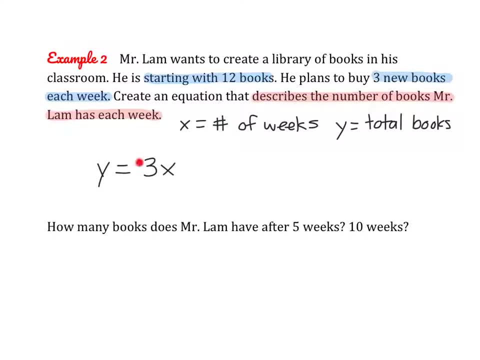 To his library, which is three X. Now this is does not represent the total number of books He has, because he started with some, So we have to add that, starting 12 on to the end. So remember the constant is always going to go right here. 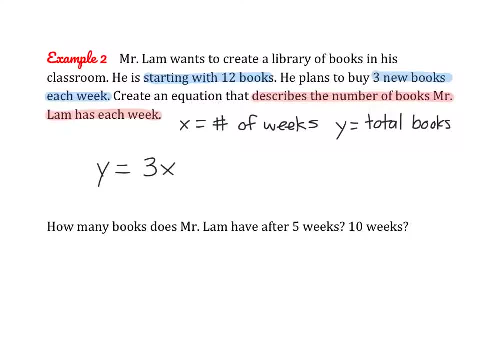 he's been adding to his list, So we can take three and multiply it by the number of books he's been adding to his library, which is 3X. Now, this does not represent the total number of books he has, because he started with some. 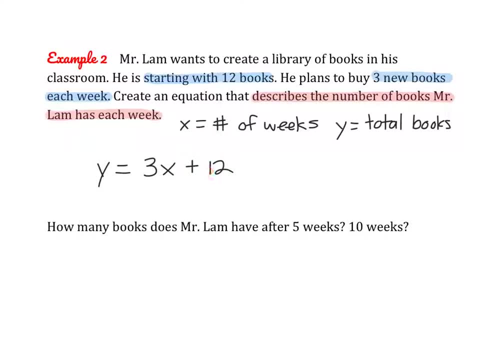 So we have to add that starting 12 on to the end. So remember, the constant is always going to go right here. So the constant is our starting point, which is 12, and our slope is always going to be how much our value is changing, and it is changing by three each week. So that's why we say 3X. 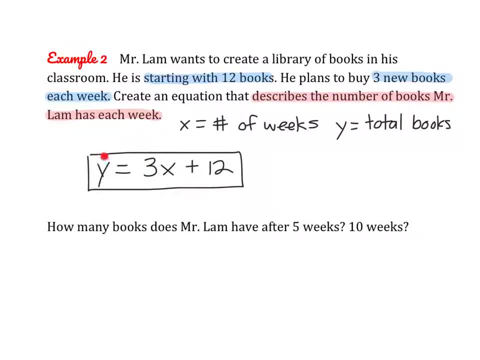 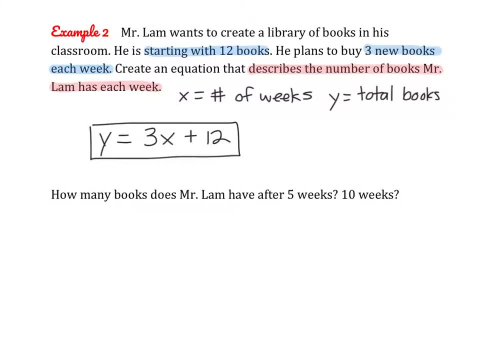 And this is the equation that can help us determine the number of books he's been adding to his list. It can help us find how many books Mr Lamb has for whatever number of weeks we want. So now let's figure out. how many books does Mr Lamb have after five weeks and ten weeks? 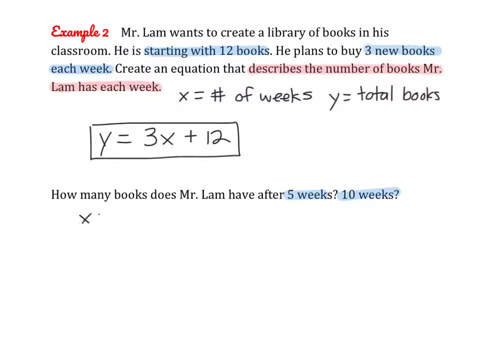 So this is the thing that we choose. So we're choosing: X equals five, an X equals 10 and we're going to substitute to solve for Y, So we have three times five plus 12.. We always multiply first, So 15 plus 12.. 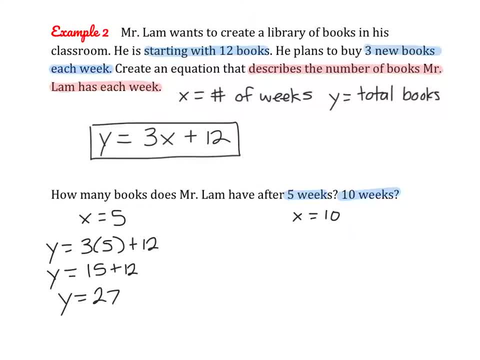 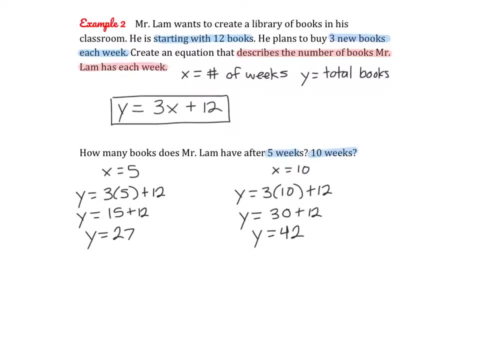 12. which is 27.. And then let's substitute: x equals 10.. 3 times 10 plus 12.. Here we have 30 plus 12, which equals 42. Now, once again, we're always going to write our final answer as a complete. 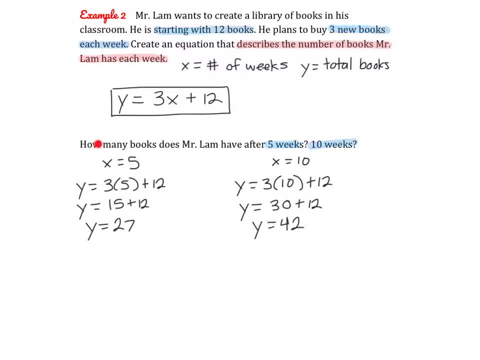 sentence and it needs to answer the question thoroughly. So how many books does Mr Lamb have after five weeks? After five weeks, Mr Lamb has 27 books, And we can do the same for the second part. How many books does Mr Lamb have after 10 weeks? We say after 10 weeks. 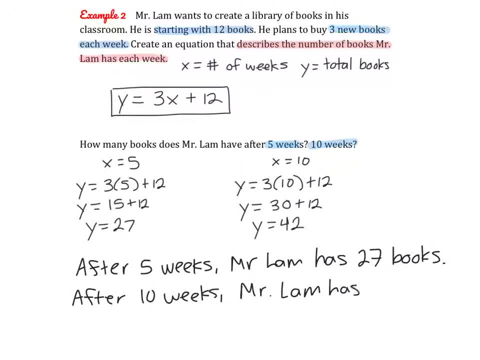 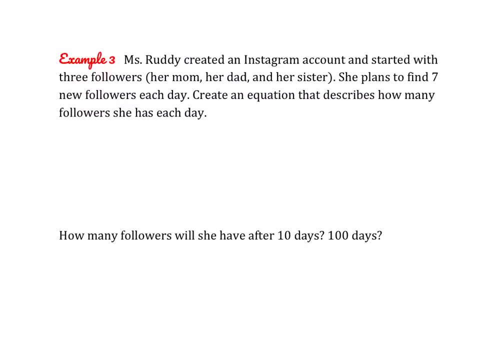 Mr Lamb has 42 books. Okay, go ahead and pause the video, and I want you to give this one a try. It says Ms Ruddy has created an Instagram account and started with three followers: Her mom, her dad. 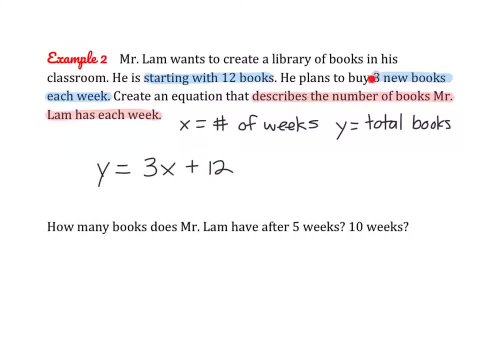 So the constant is our starting point, which is 12.. And our slope is always going to be how much our value is changing, And it is changing by three each week. So that's why we say three, X, and this is the equation. 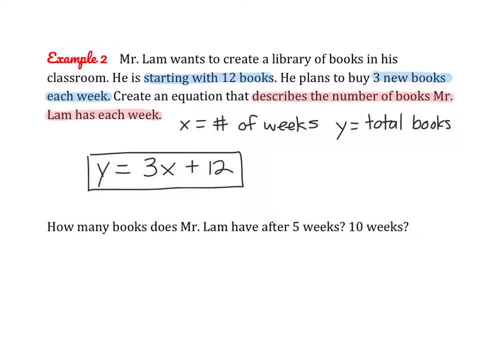 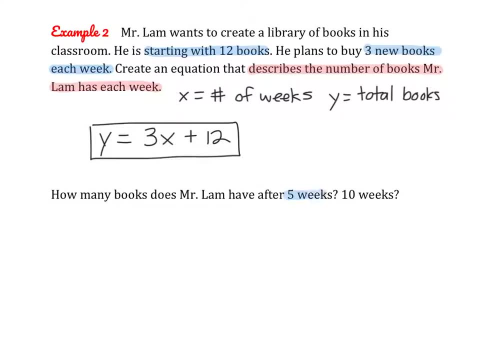 That can help us find how many books Mr Lamb has for whatever number of weeks we want. So now let's figure out how many books does Mr Lamb have after five weeks and 10 weeks? So this is the thing that we choose. 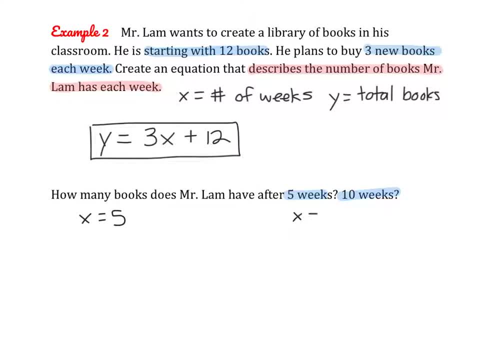 So we're choosing: X equals five and X equals 10.. And we're going to substitute to solve for Y, So we have three times five plus 12.. We always multiply first, So 15. Plus 12, which is 27.. 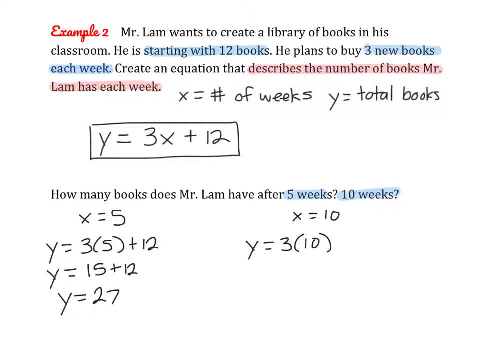 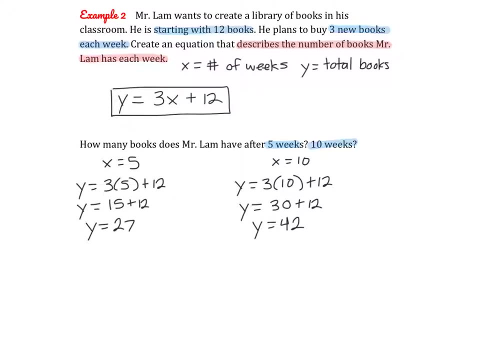 And then let's substitute: X equals 10, 3 times 10 plus 12.. Here We have 30 plus 12, which equals 42. Now, once again, we're always going to write our final answer as a complete sentence. 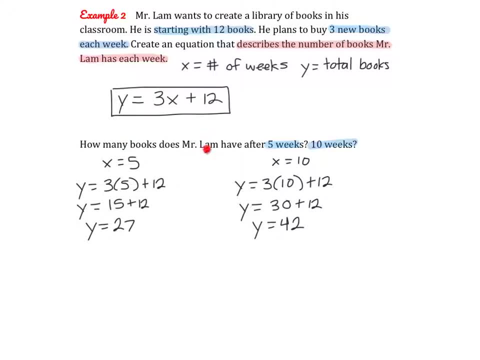 And it needs to answer the question thoroughly. So how many books does Mr Lamb have after five weeks? After five weeks, Mr Lamb Has 27 books, And we can do the same for the second part. How many books does Mr? 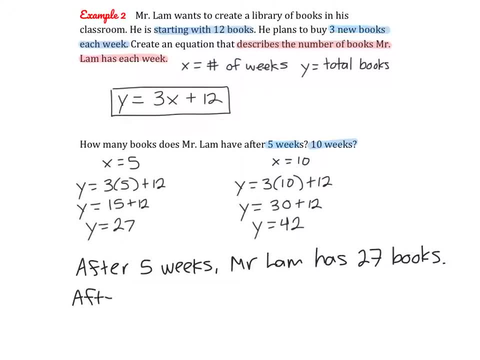 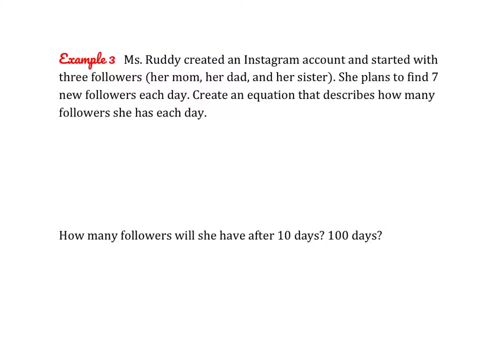 Lamb have. after 10 weeks, We say After 10 weeks, Mr Lamb Has 42. Books. Okay, go ahead and pause the video, and I want you to give this one a try. It says: Miss ready has created an Instagram account and started with three followers. 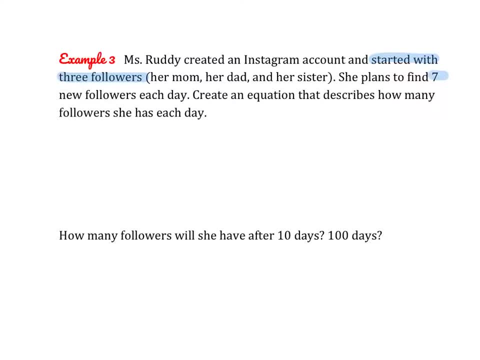 Her mom, her dad and her sister. She plans to find seven new followers each day. created equation that describes how many followers she has Each day. So go ahead and pause the video and make sure you're using your desk: Define, make an equation, solve and complete sentence. 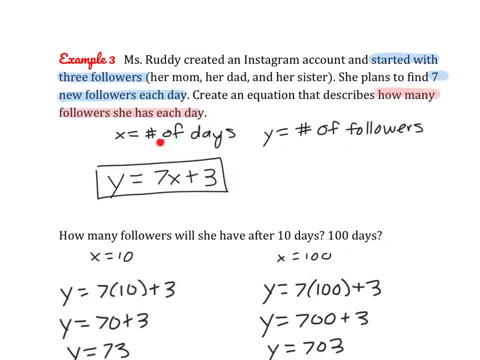 All right, let's go ahead and check. So here, X is going to represent the number of days, because that's the only thing that we can pick and choose, and why is going to represent what we're trying to find, which is how many followers.